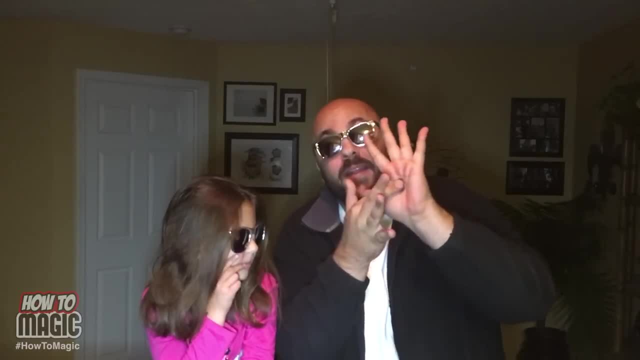 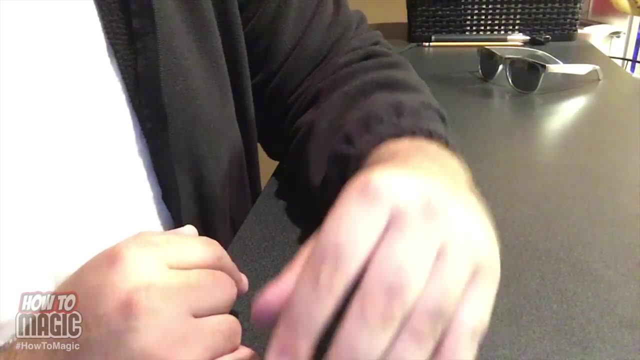 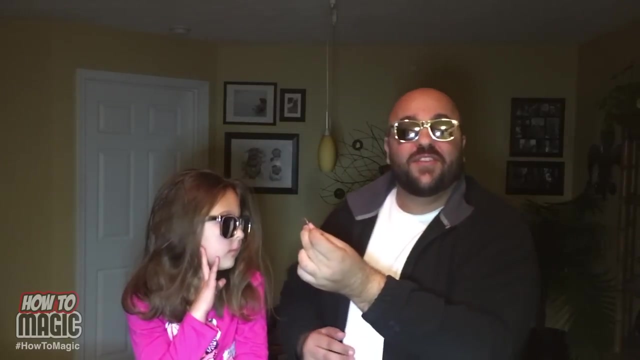 Alright. So you take the quarter and you palm it in your hand. And what palming is is you conceal it in your hand and make your hand look natural so that nobody knows the quarter is in your hand. And then you just reach up, pull the quarter out of your palm and make it look like you just pulled it right from behind their ear. 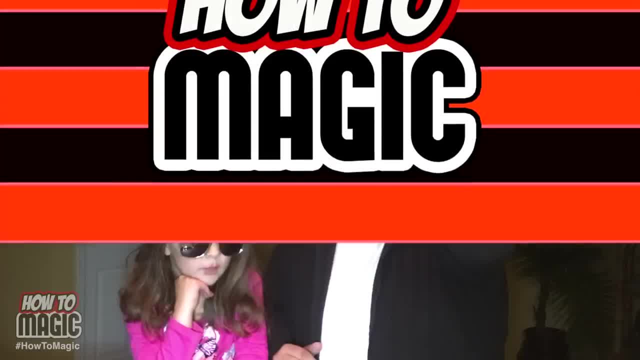 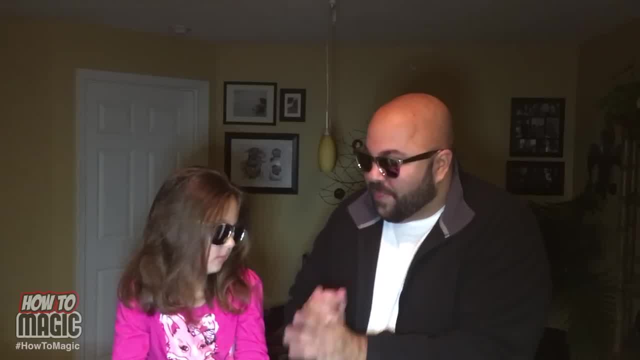 And that is how you do the magic coin from the ear trick. Alright, guys, this one is a classic magic trick that you can do with just your hands. I take my hands like this and I'm going to grab onto my thumb like this: 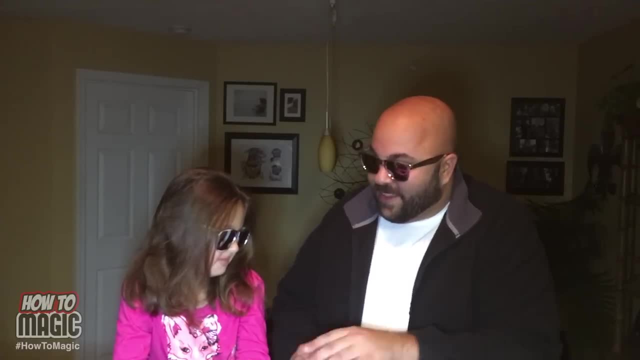 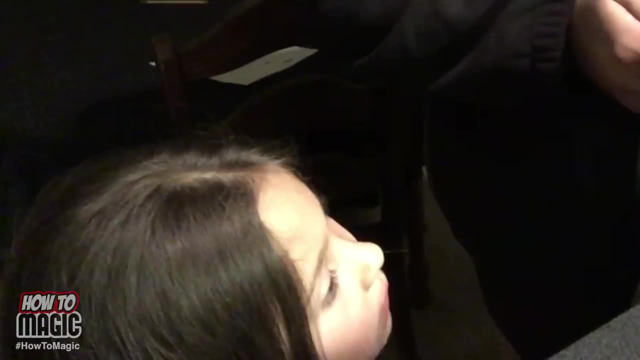 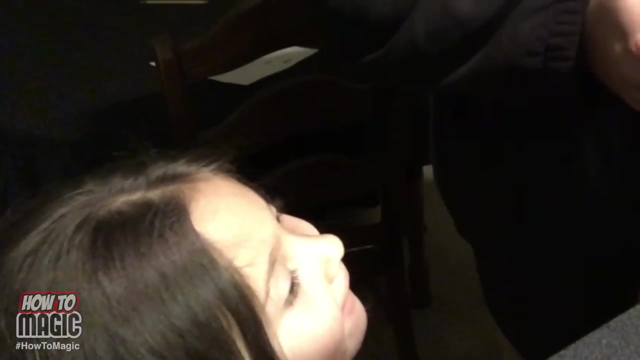 And I'm going to try and pull my thumb off my hand. You think I can do it? Uh-huh, You think I can Really. Alright, let's see. Watch, Isn't that good? Watch? You want to tell them how it's done? 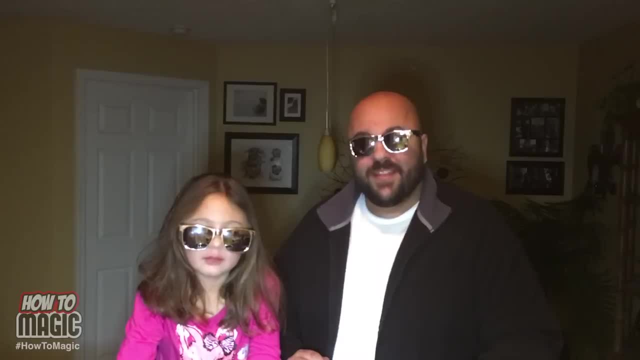 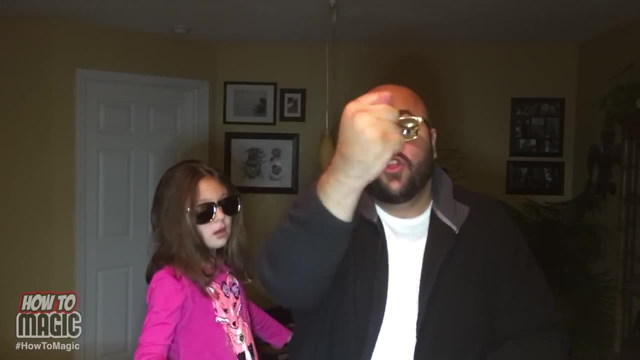 No, We shouldn't tell them. No, I think we should tell them. They probably want to know. Here's how it's done. All you do is take the thumb of your other hand and make it look like it's this thumb. 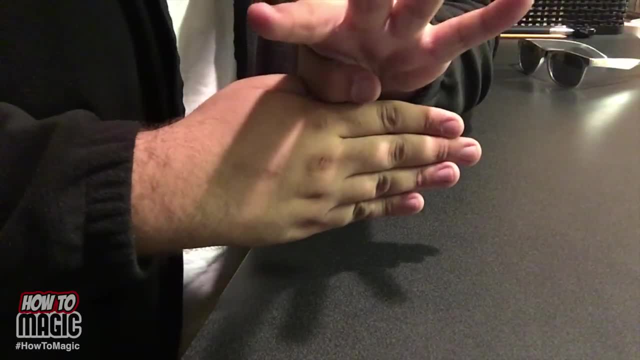 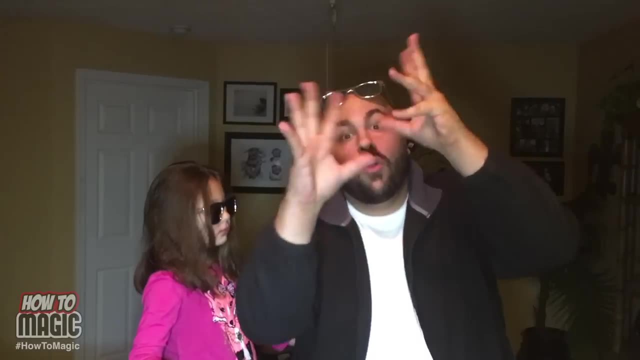 So you bend this thumb down and at the same time this one comes up and it looks like your thumb is just severed. And that's how you do the magic thumb trick. On to the next one. It is a jello pencil. You ever seen a jello pencil before? 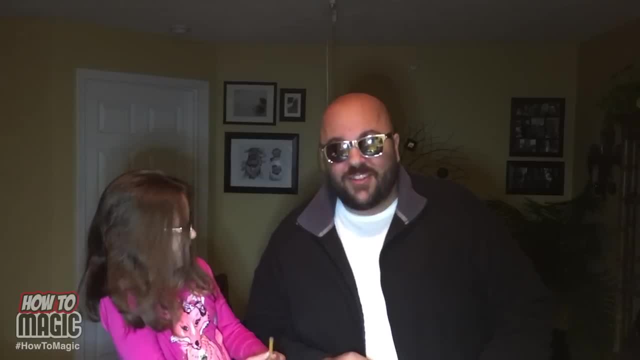 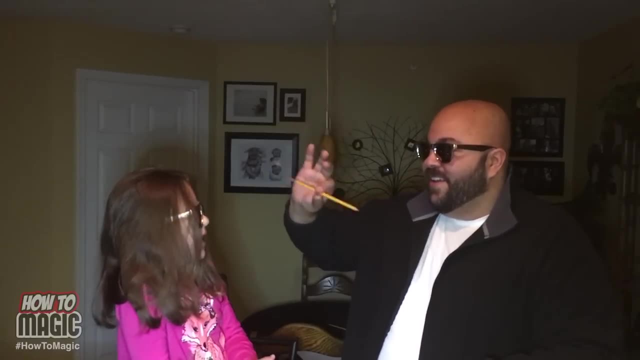 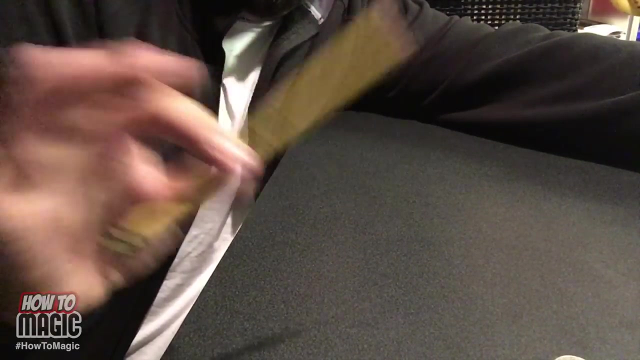 Here. feel it. Can you feel it? It's jello. What Look? It looks like jello. It's like a spider Watch, Doesn't it look all wavy like jello Watch? It starts to just look like it's waving like that. 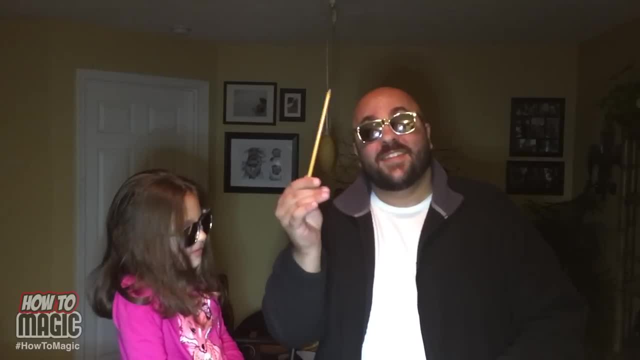 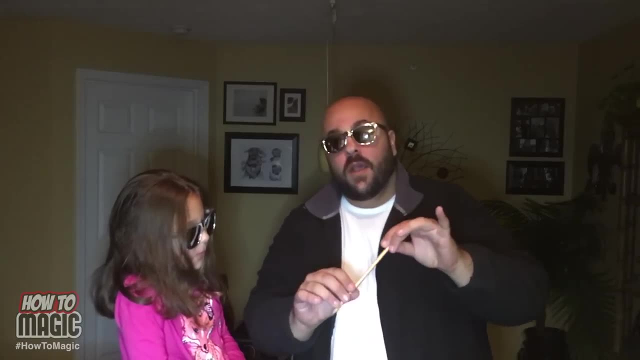 Isn't that cool. Alright, guys, this is a classic trick. It's actually an optical illusion. The way this works- and, Ava, you probably don't even know this either. this is actually the first time I've explained it to you. when you wave the pencil like this, you hold your fingers lightly. 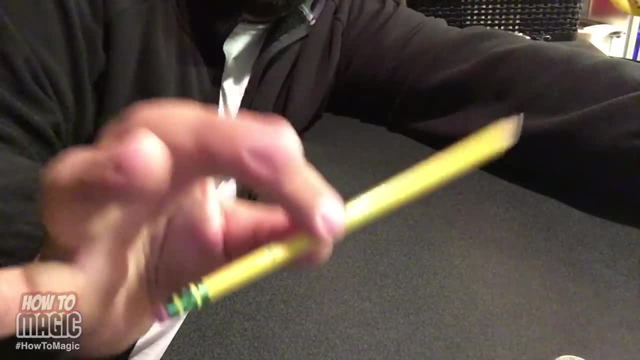 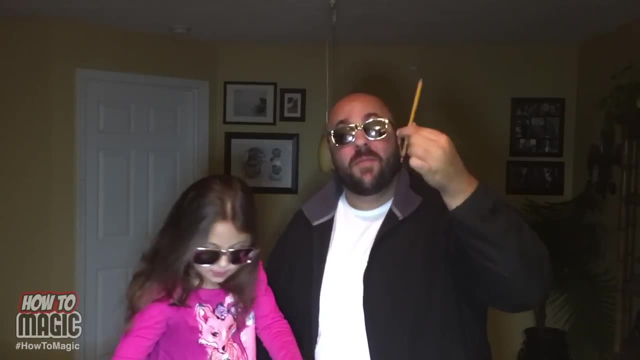 and just wave it back and forth, and it creates this optical illusion that the pencil is made of rubber and it looks like it really is just bending like that, doesn't it? so that's how you do the magic rubber pencil trick. where are you going? all right, this next. 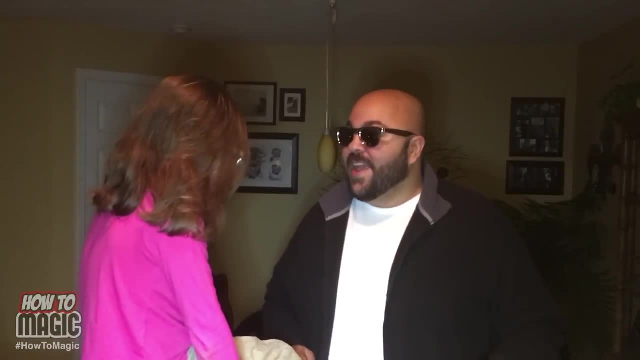 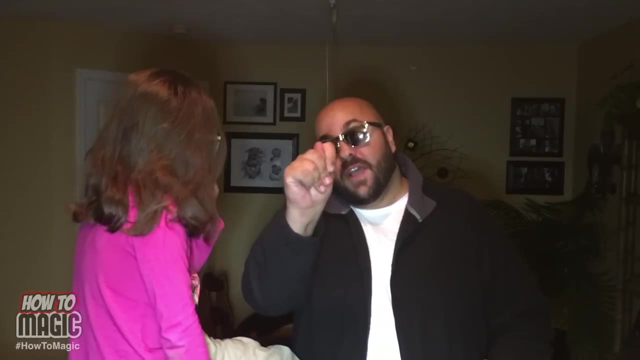 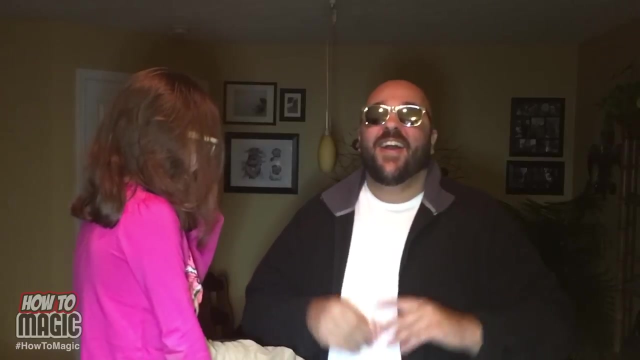 one's a classic magic prank. here's how it goes. hey, ava, i got your nose. you're right, i didn't really have your nose, it was just my thumb, but this time i really got your nose. all right, guys, this one's simple. all you need is one of these fake. 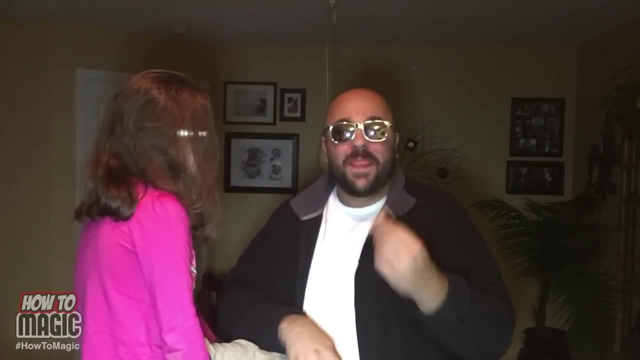 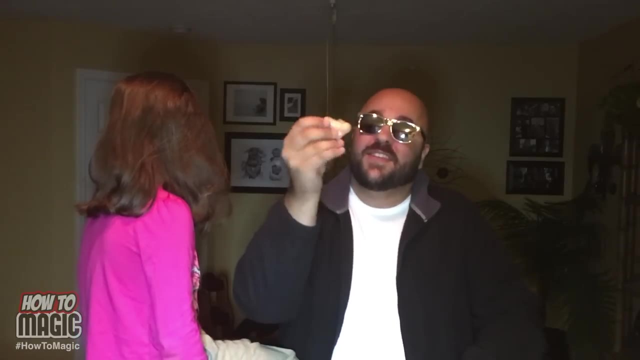 plastic noses. you can get these online or at a magic shop and you can do the original got your nose trick by just putting your thumb in between your fingers like this, and then you can step it up a notch and get yourself a plastic fake nose and really freak out your kids or your friends or your 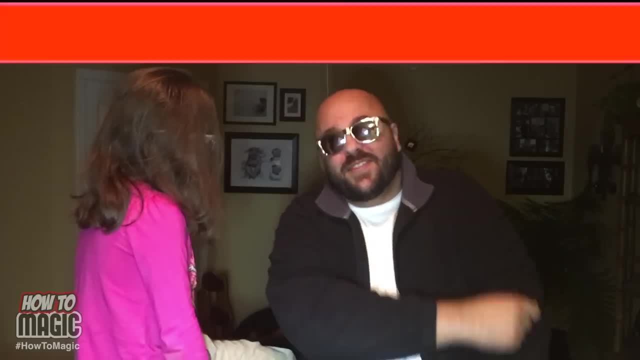 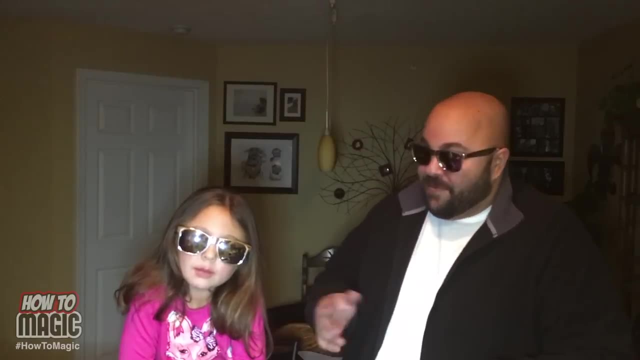 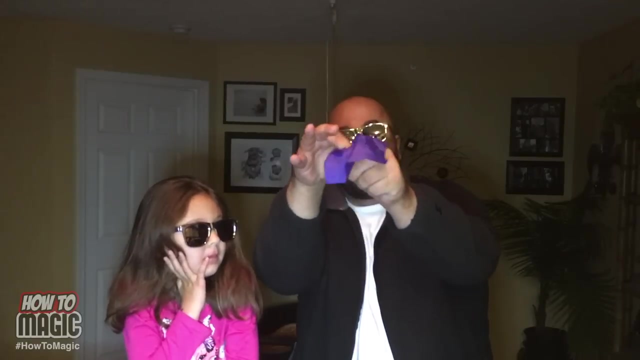 family or your classmates. have fun with it. on to the next one. all right, guys, this one is a classic magic trick that will absolutely amaze people. here's how it goes: ava, will you please present us with our prop- a beautiful blue scarf- and it goes right into our hand, just there. 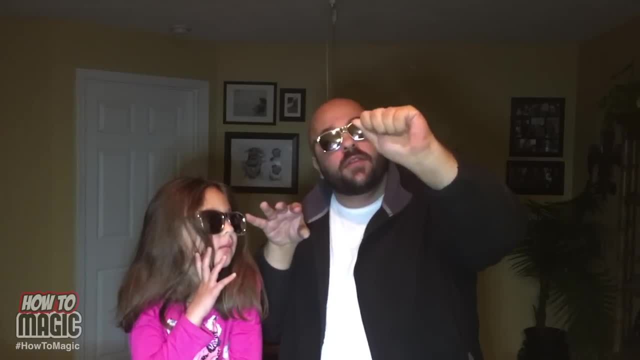 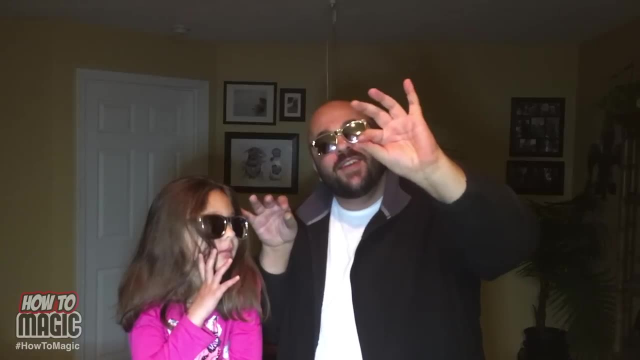 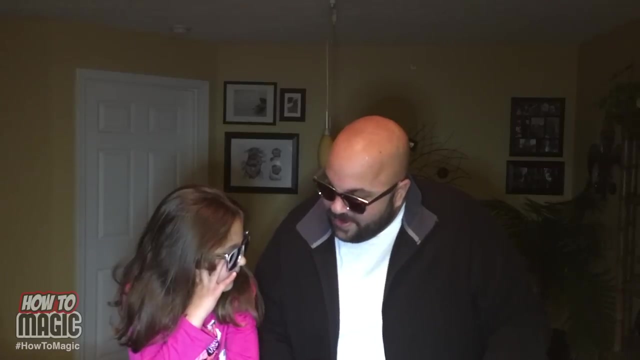 stays inside the hand and we rub it. we just rub a little bit, get a feel for it and then, as we rub, it just just slowly starts to disappear until it's completely gone. isn't that cool? yeah, but where is it? i know? don't you want to know where it is watch? 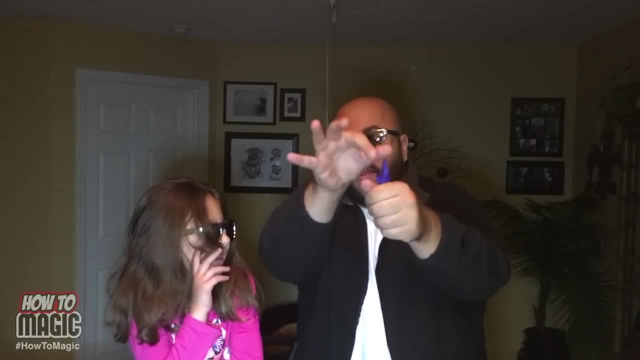 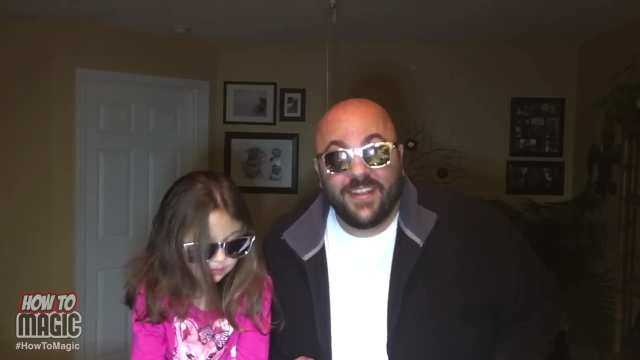 it's in your pocket. no, watch, that's not in my pocket, it's actually right back here. you guys want to learn how it's done. i'll show you how it's done in view right now. all right, guys, that's it for this video. i hope you enjoyed it and i'll see you in the next one. bye, bye. 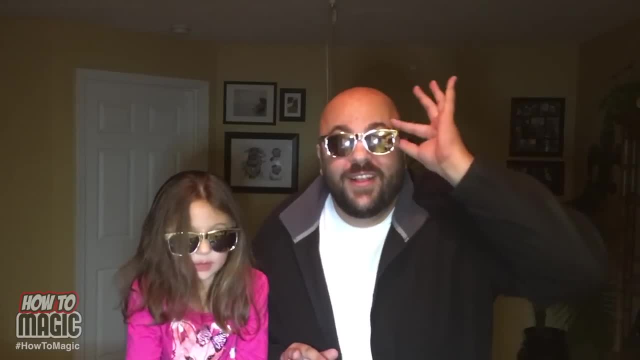 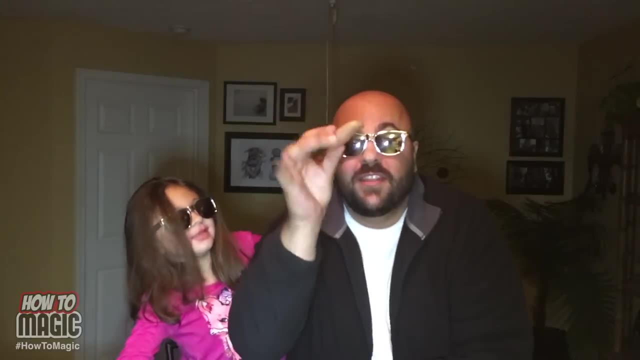 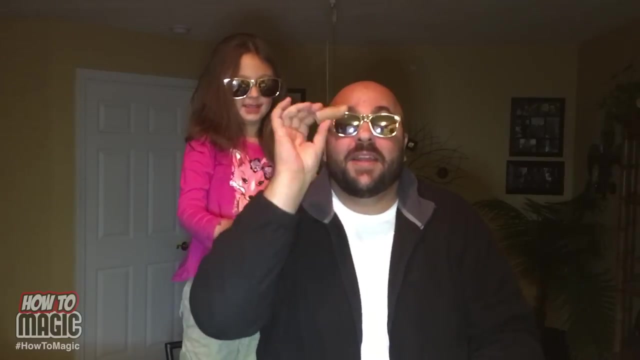 all right, here's how it's done. i'm about to reveal the secret, all right. so this is the secret. it's a plastic thumb tip. you get these at a magic shop or online and this: you also need one of these. i'm gonna give this away at the end of the 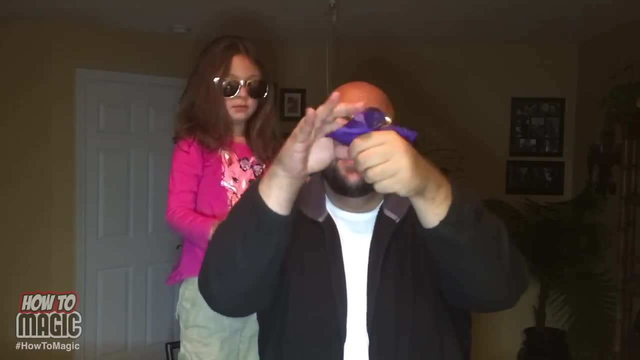 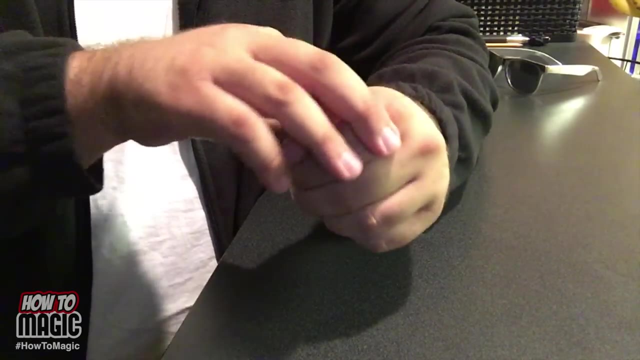 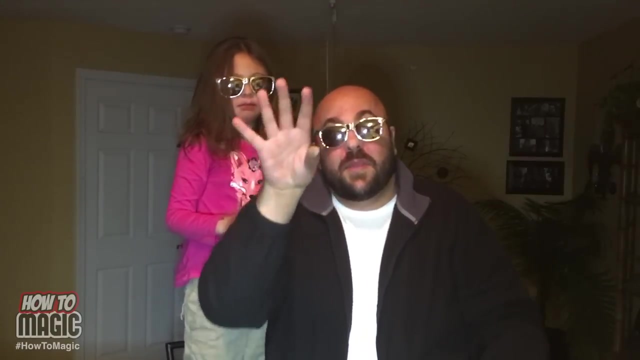 video. so stay tuned. you take this thumb, conceal it in your hand. the sash goes inside. you're not photo bombing me, are you inside? thumb goes inside. all the attention is over here on this hand. you make it disappear. keep your thumb tip pointed towards your audience, if you.